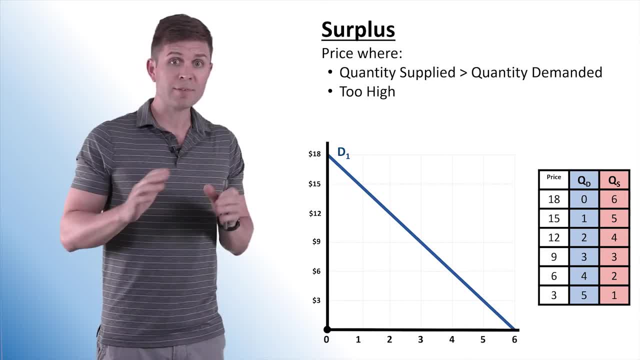 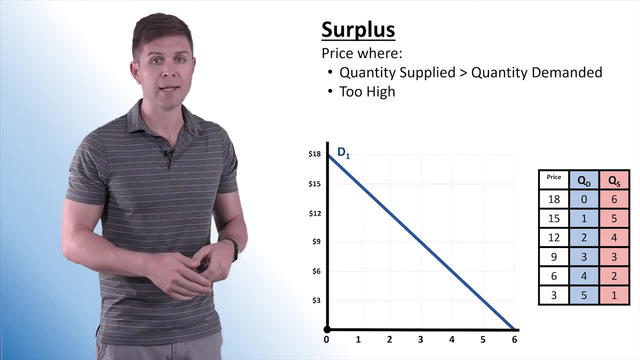 markets usually end up in equilibrium, But sometimes it takes a little time to get there. In some cases we end up with a surplus. A surplus is when the quantity supplied exceeds the quantity demanded. There's extra product on the shelves. Price is usually too high. 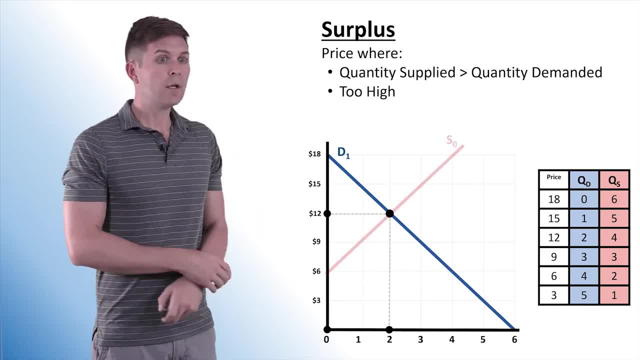 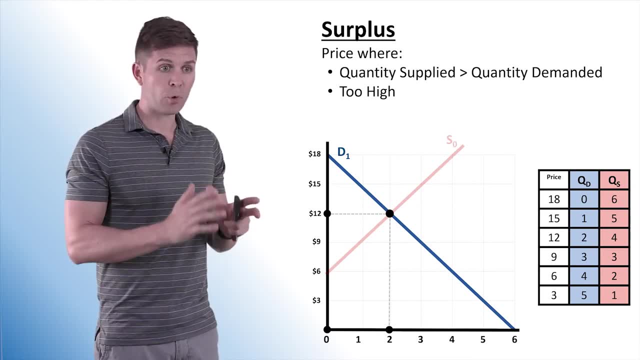 and will eventually come down. But let's see how this gets started. So let's imagine that originally this is our setup. We have an equilibrium price of $12, quantity supplied, quantity demanded are both $2 at this point, And then something changes. Supply shifts to the right. We have, let's say, 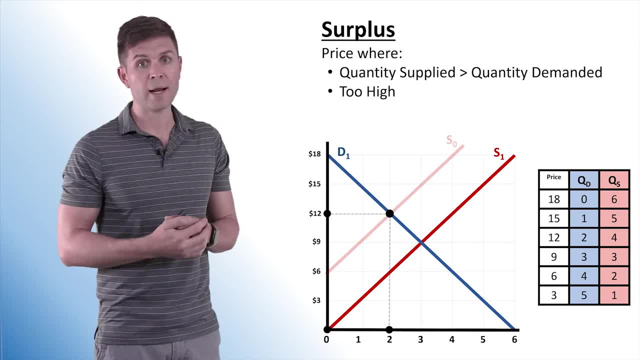 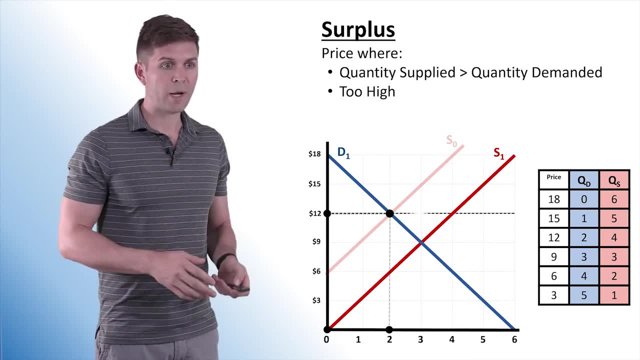 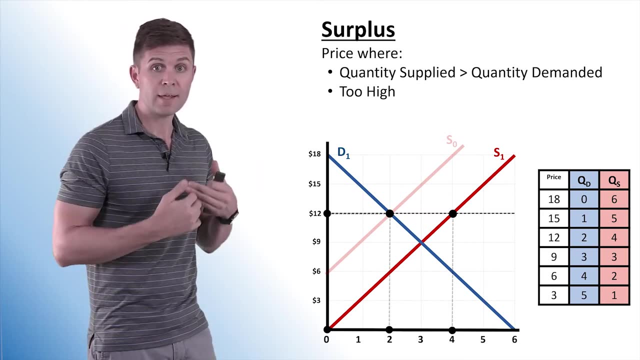 a drop in input prices and suppliers can produce more at every price level. It doesn't automatically change in the market. It takes a little time to adjust. So in this situation we're going to continue at that $12 price level. Suppliers are happy to supply more at $12 and they can because 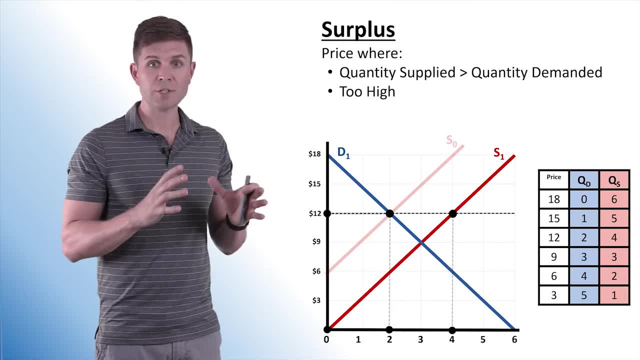 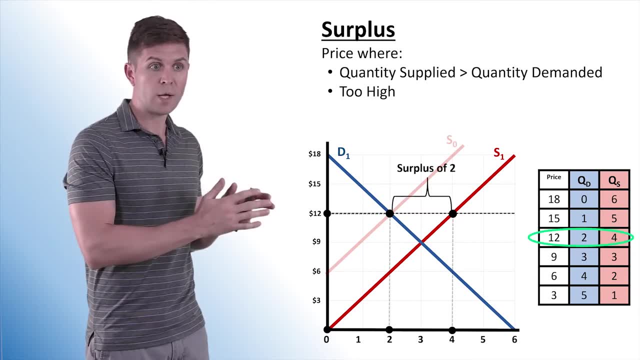 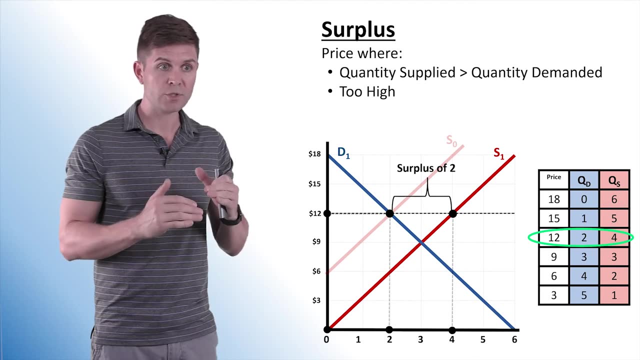 input prices are cheaper, But consumers, they're not changing at all. They're still stuck at that $12 price level. So the quantity demanded in this situation is 2.. The quantity supplied is 4 and we have a surplus of 2 units. Now eventually, as markets will adjust, 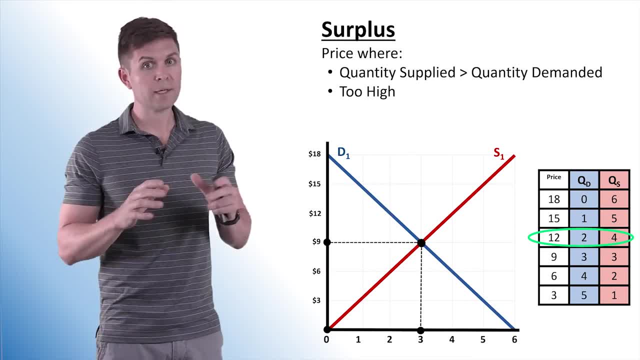 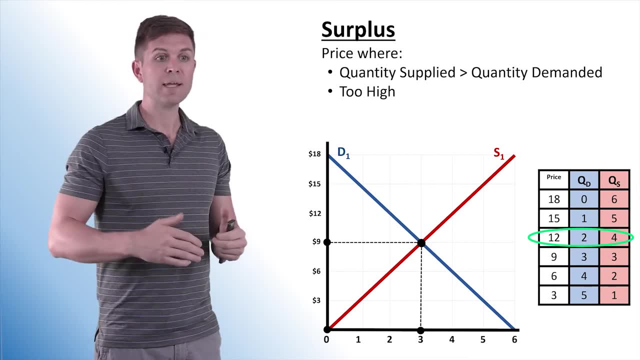 price level will come down. The producers will say: we need to get rid of this extra product. Let's drop the prices a little bit. And that drop in price will sell to more consumers and at the same time will discourage producers from producing as much. And then we find our new equilibrium at 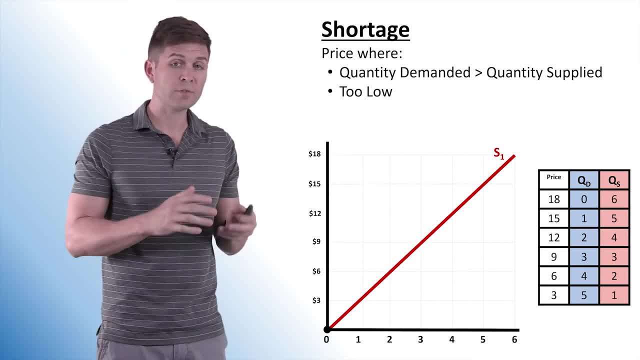 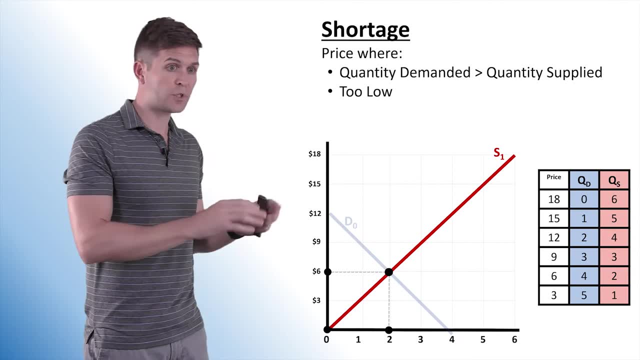 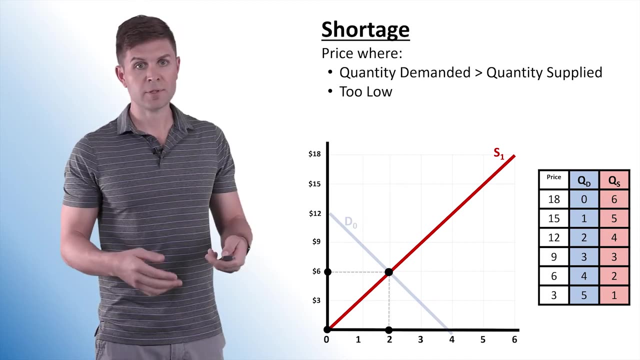 $9 once again. Under other circumstances, when price is too low, we end up with a shortage. This means that the quantity demanded is higher than the quantity supplied. So let's start with this original model: At $6, our quantity demanded is 2, our quantity supplied is 2.. We are in equilibrium. and then something. 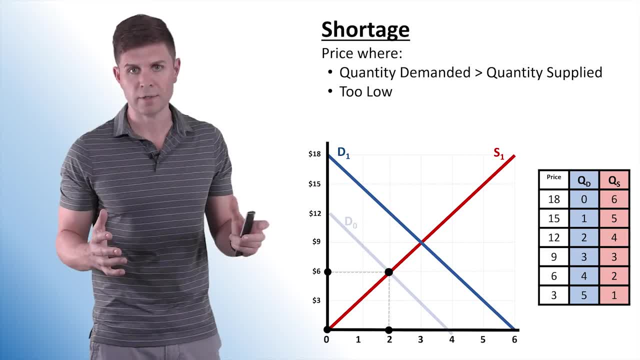 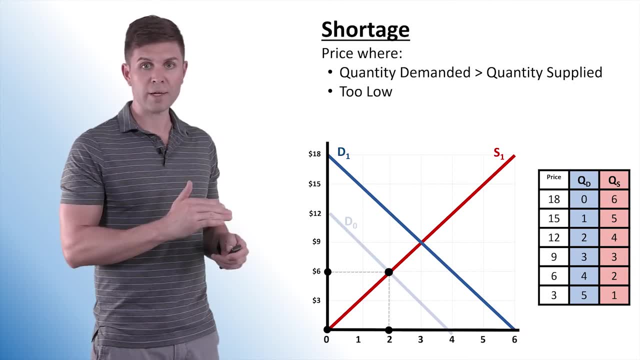 changes. Let's imagine that demand increased because of consumer taste changes. So we have a new equilibrium that should be established. but we're not quite there yet. We're still operating under the old price level. it hasn't quite adjusted. Under this we see that the quantity demanded is going to be. 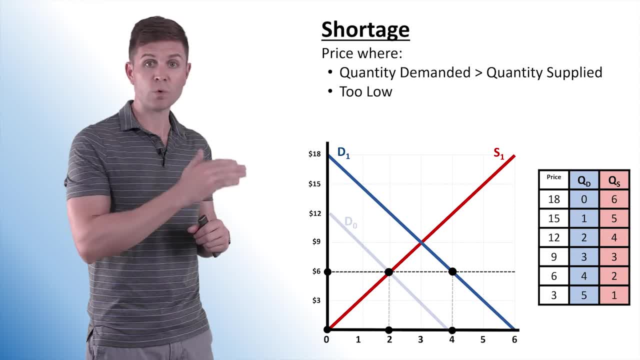 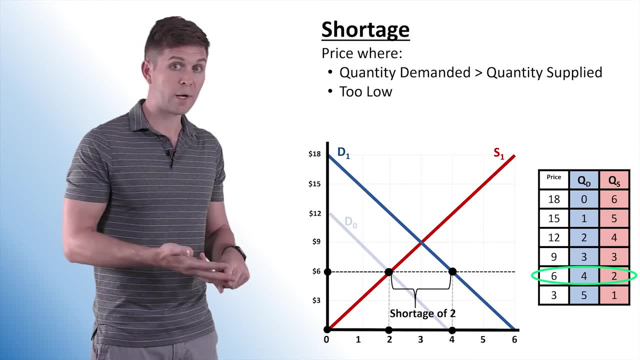 much higher. it's going to be to 4, but price hasn't changed yet, so quantity supplied stays the same. So in this case we have a shortage. we have a quantity demanded of 4, which exceeds the quantity supplied of 2, giving us that 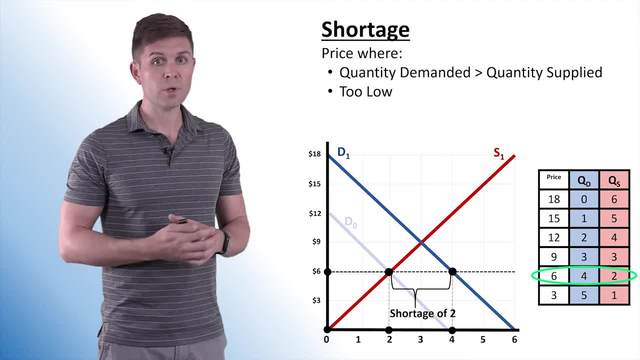 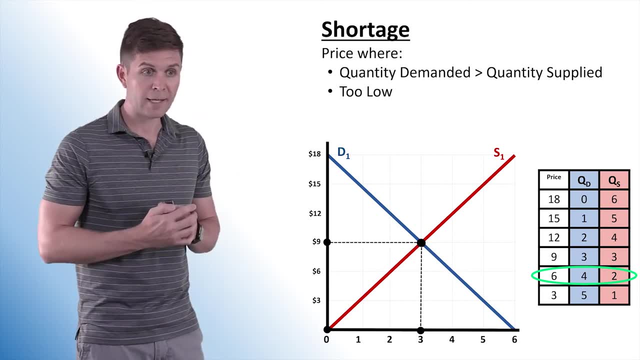 shortage of two units. Eventually, producers will understand that they can raise the price a little bit and in doing so, that discourages purchases. buyers will buy a little bit less and producers will produce a little bit more, increasing the quantity supplied, decreasing the quantity demanded and 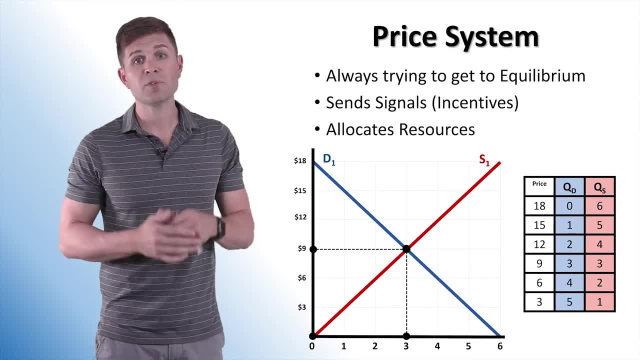 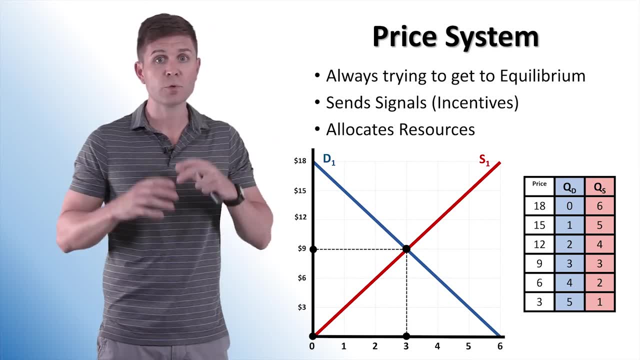 getting us back to that equilibrium one more time Now. the price system is always trying to get back to equilibrium- equilibrium And it's using that invisible hand to help guide resources and convince producers and consumers to do what it needs to do. It sends signals in the form of prices to consumers. 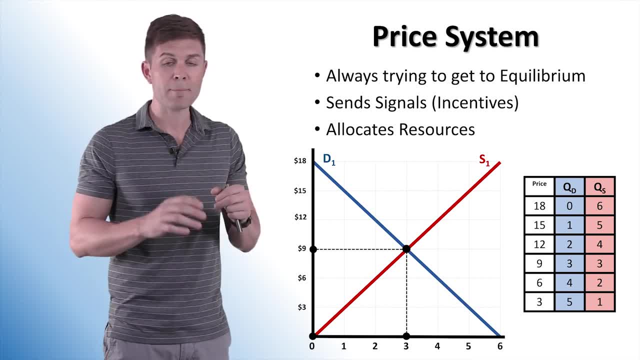 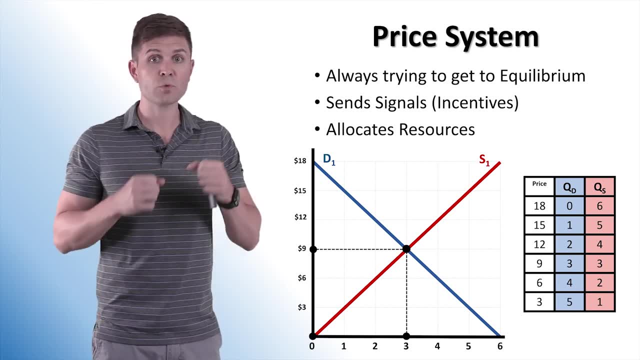 If price is too high, they buy less. If price is too low, they buy more, And producers respond to this as well. Everybody's an optimizing individual. As prices change, consumers and producers will do what's in their best interest, And it always pushes that price back to equilibrium And in 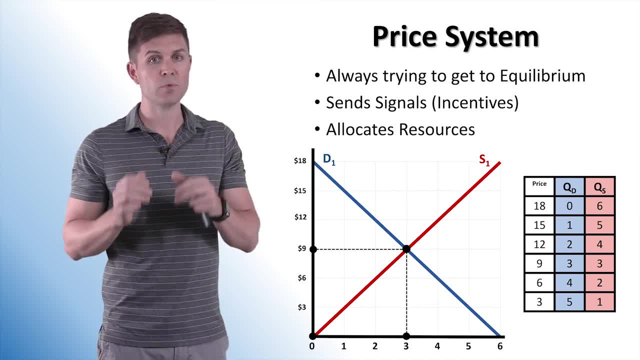 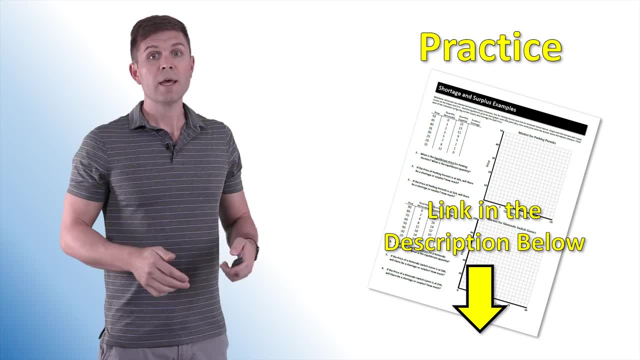 doing so, it allocates resources by providing them to the people who value them the most. All right, make sure you're checking out the practice assignment that you can find in the link below down in the description And, in addition, make sure you check out the. 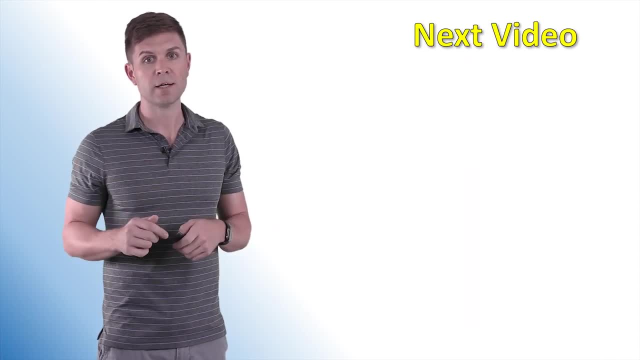 next video in this series. As always, thank you guys for watching and I'll see you next time. 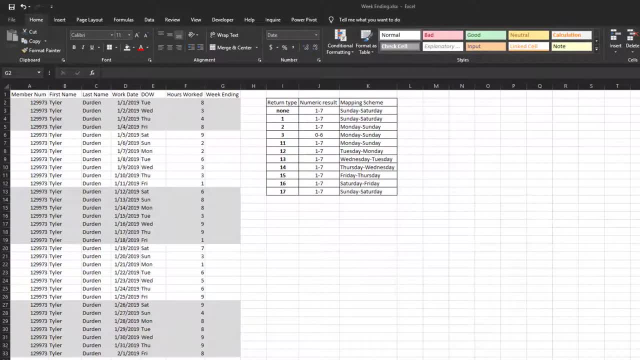 Welcome to Single Serve in Excel. Today we're going to create a week ending date. There are times when you need to create a week ending date based on some work date in order to group a work week. Let's say you work for a company where the work week ends on a Friday. 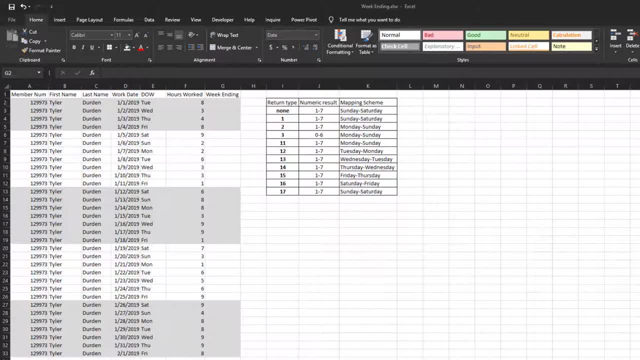 So that means the first work day of the week is a Saturday and the last work day of the week is a Friday. In our example, Tyler works seven days a week for the entire month. The shaded and non-shaded areas represent a work week. This is just there to help you see the grouping by week.